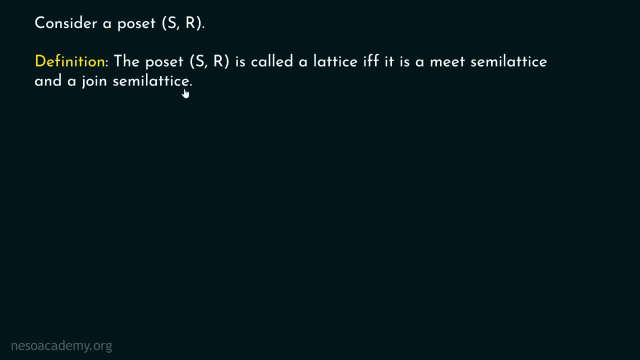 is a mid-semi-lattice and a joint semi-lattice or not. Okay, Let's see one example to better understand. this Is the given hash diagram, a lattice. That is the question. This is the hash diagram available in front of us. We have to determine whether this wallet is a 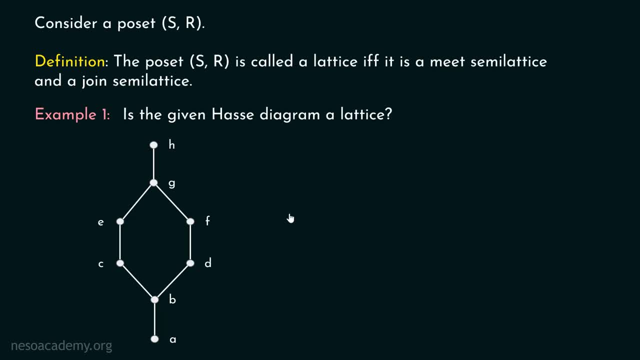 lattice or not. Let's consider the solution of this particular example. We know that a has diagram is called a lattice if it is both Mid-semi-lattice and joint semi-lattice. So for the hash diagram to be a lattice, it must be a Mid-semi lattice and joint semi-lattice. 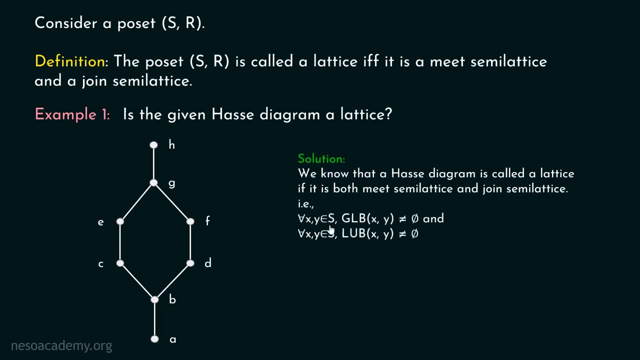 Okay. In other words, we can say for all: x comma y belongs to S, greatest lower bound of x comma y mit 32.5 minus 2 times. Dream is not a lattice. If S comma Y belongs to S, then we are not LET安全 a hatchet toف. 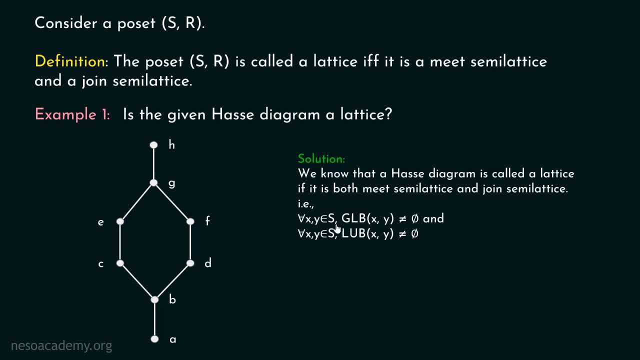 We can follow this siemens to find out whether that phase at norm is a lattice. If S, comma, y, middle reducing must not be equal to phi. This is the definition of mid-semi-lattice. We must consider every pair of set S. 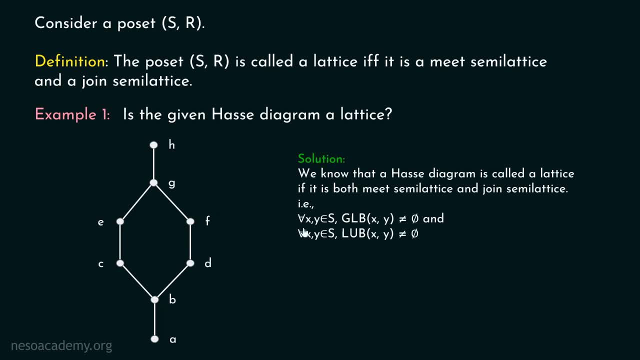 Here I am considering as a poset, For all belongs to S greatest lower bound of must not be equal to phi, And for all belongs to S least upper bound of must also not be equal to phi. This is the definition of joint semi-lattice. 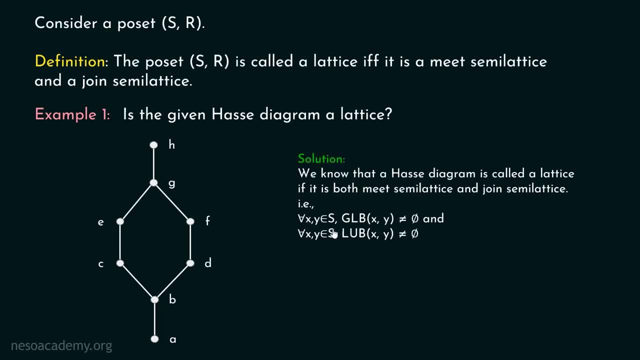 So mid-semi-lattice and joint semi-lattice must be satisfied. Then only we can say: a hash diagram is called a lattice. Now consider the incomparable pairs. Obviously here I am talking about every pair, But better is to consider the incomparable pairs. 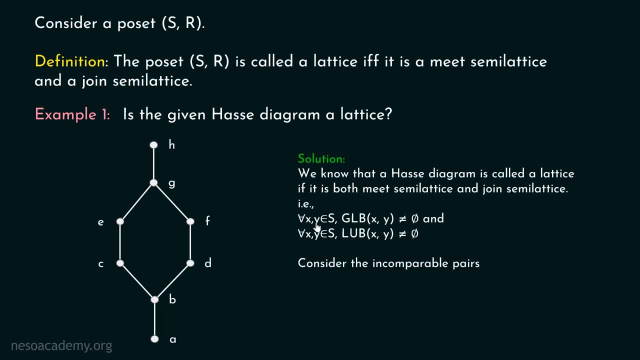 because for the comparable elements, greatest lower bound and least upper bound must always exist. That is why it is important to consider incomparable pairs. Let's consider all the incomparable pairs in this hash diagram. You can see E and F are incomparable. 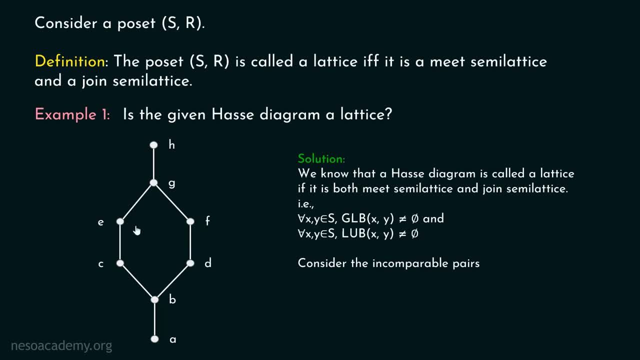 Let's find out the greatest lower bound and least upper bound of E and F. Greatest lower bound of F, E or E, F- they both are same- is actually equal to B. Right, You can see that greatest lower bound of E, F is B. 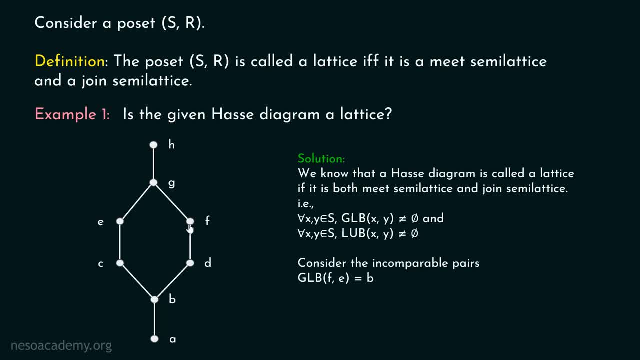 We have to trace the path down from these two vertices, And here we have to see where they meet. They meet at this point right. This is the first point where they meet. Therefore, this is the greatest lower bound of F? E. 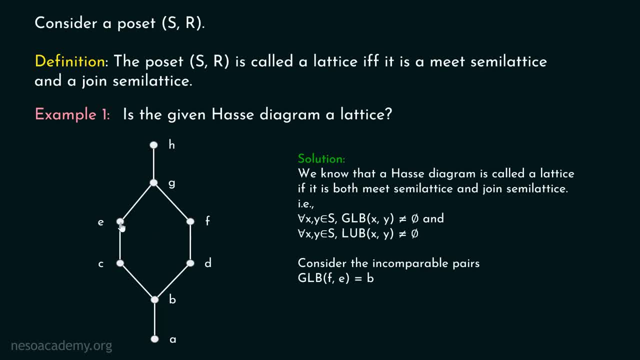 Now let's identify the least upper bound of F? E or E F. Least upper bound of F? E is equal to G. You can see that they meet at this point. Obviously, we have to trace the path upwards, right. 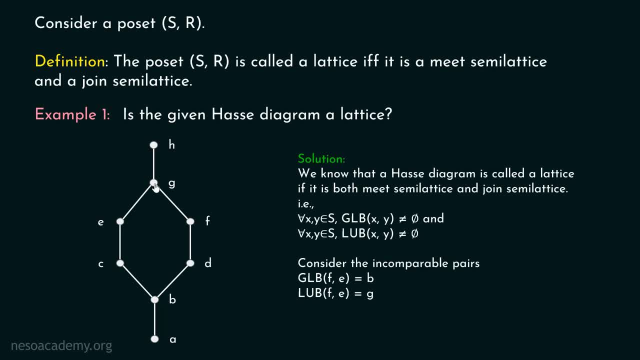 You can see that they meet at this point. This is the first point where they meet. Therefore, this is the least upper bound of F- E. Now we will see the least upper bound and greatest lower bound of C and D, because these two are incomparable as well. 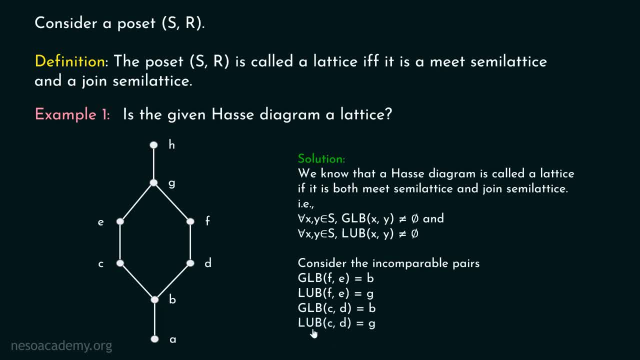 Greatest lower bound of C D is B and least upper bound of C D is G. You can clearly see this: Greatest lower bound of C D is B and least upper bound of C D is G. Right, Then we will find the greatest lower bound of E and D. 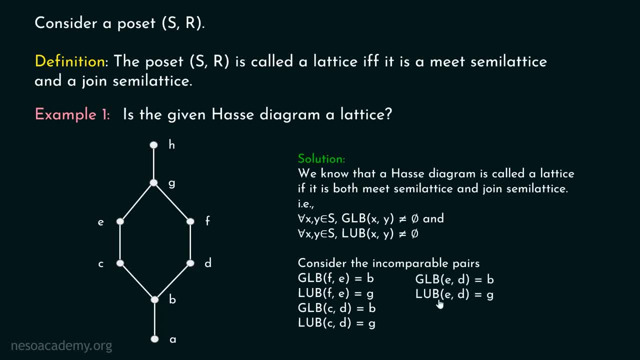 Okay, Greatest lower bound of E- D is B and least upper bound of E and D is G. Right Again, greatest lower bound of E D is B- They meet at this point- And least upper bound of E- D is G. 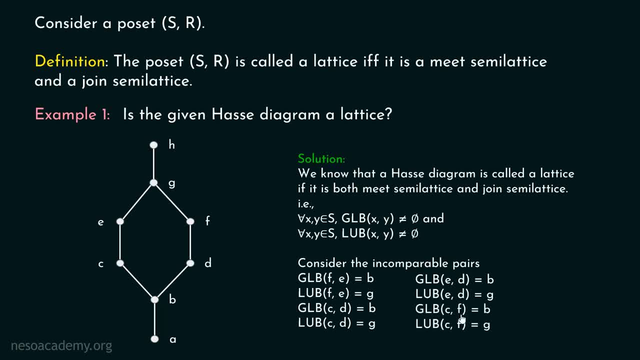 Similarly, greatest lower bound of C F is B and least upper bound of C F is G. You can see, for every incomparable pairs- greatest lower bound and least upper bound- do exist. Therefore, the given Hess diagram is a lattice. 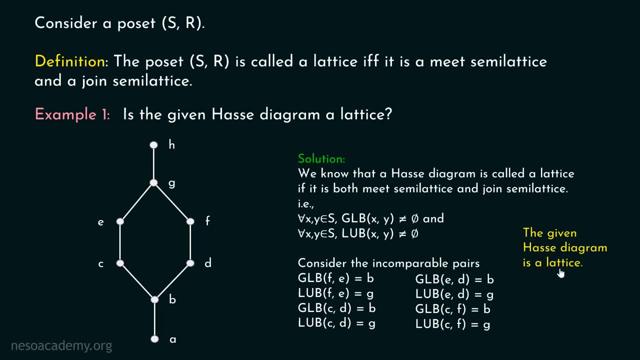 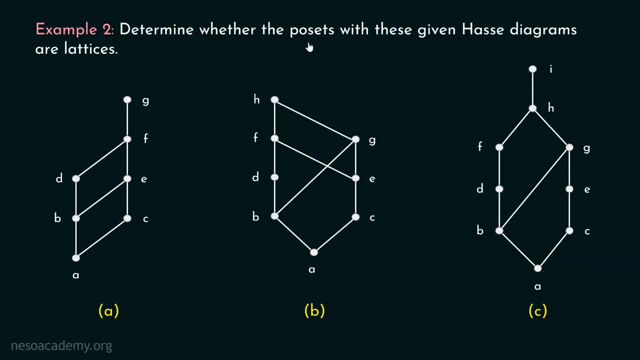 Fine, There is no doubt about this, that this Hess diagram is a lattice. Okay, Now here is example two. Determine whether the post sets with these Hess diagrams are lattices. These are the available Hess diagrams in front of the screen. 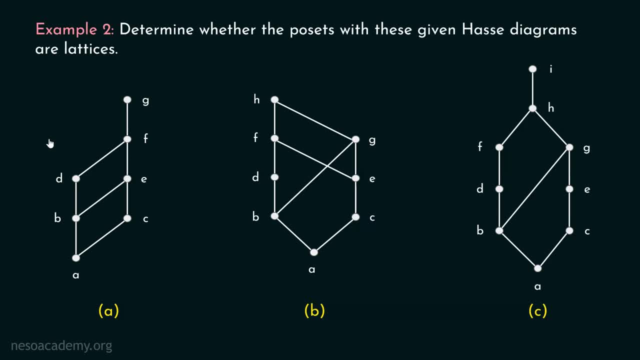 Now our job is to determine whether the post sets with these given Hess diagrams are lattices or not. Okay, Let's consider this particular Hess diagram first. Here we have to determine whether this Hess diagram is a lattice or not. Consider the pair D, E. 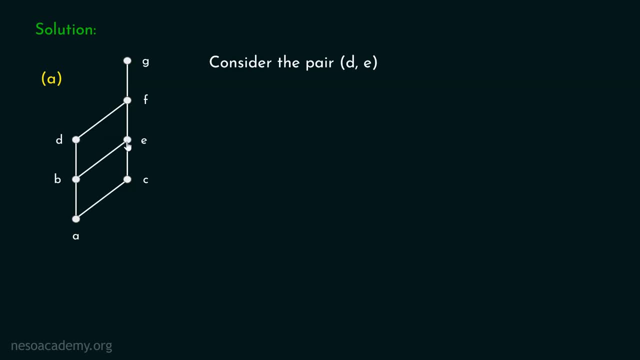 Let's consider these two elements. We have to see the incomparable elements. You can see that these two are incomparable elements. Right, Let's consider these two elements. We have to find the greatest lower bound and least upper bound of these two elements. 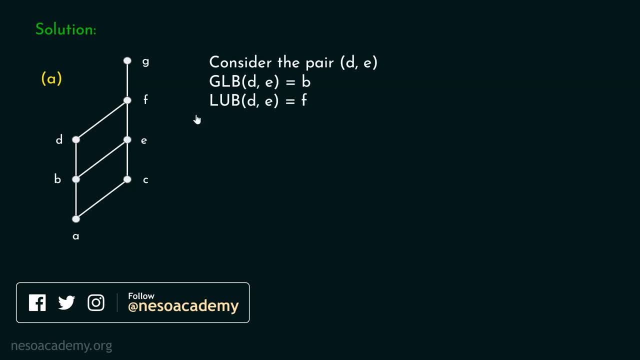 Greatest lower bound of D? E is B. You can see that greatest lower bound is B And least upper bound of D? E is F Right. Similarly we can consider the pair B- C, And for these two elements the greatest lower bound is A and least upper bound is E. 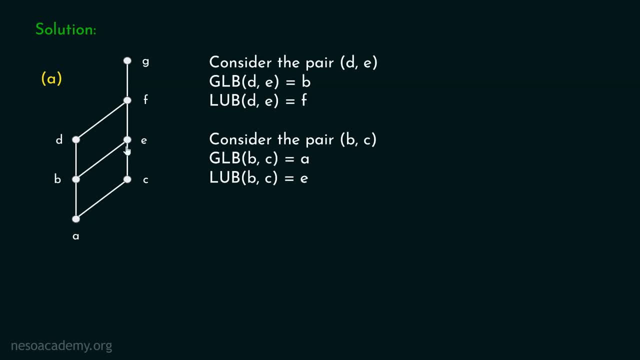 You can see, the greatest lower bound is A and least upper bound is E. For every pair of elements, especially incomparable elements, the greatest lower bound and the least upper bound exists. Therefore, the given Hess diagram is a lattice. There is no doubt about this, that this Hess diagram is a lattice. 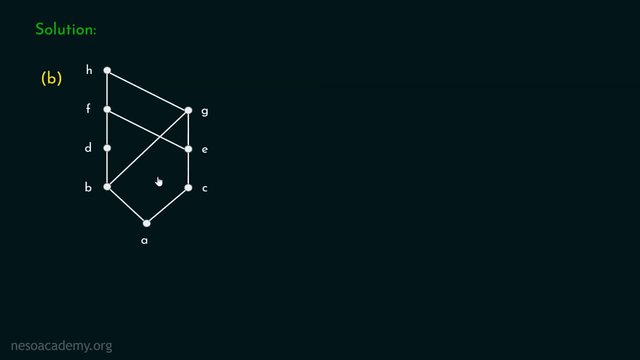 Okay, Let's see figure B. Is this a lattice? Okay, Let's consider the incomparable elements. Consider the pair F- G. Let's consider these two elements, F and G. Fine, Let's find the greatest lower bound and least upper bound of these two elements. 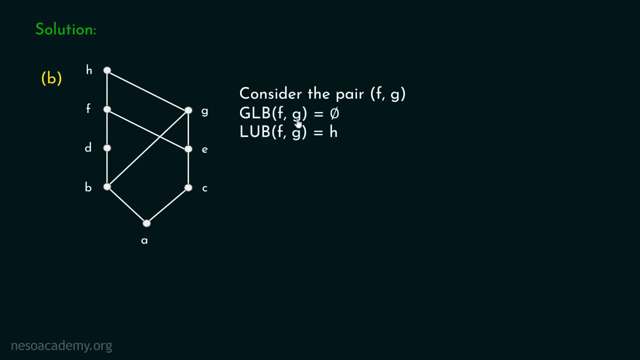 You can see that the greatest lower bound of F? G is Phi And least upper bound of F G is H. Why is that so? You can see that the first meeting point of F? G is E as well as B. These two are the first meeting points. 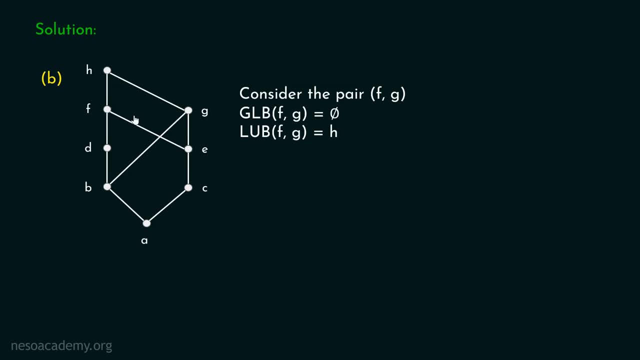 There is no single first point where these two points meet. Right, If we trace the path down, we can see that they meet at this point as well as this point at the same time. Right, These two are the first meeting points. Therefore, greatest lower bound of F G does not exist. 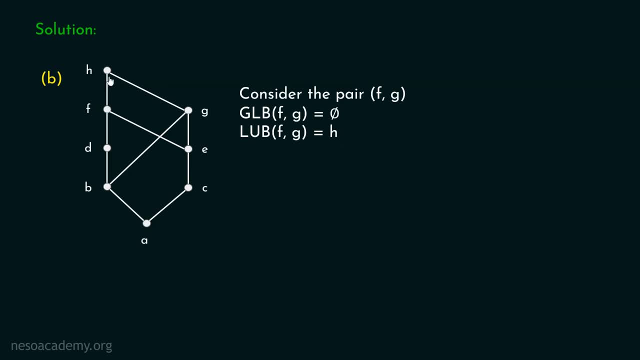 But least upper bound of F- G is H. You can see that least upper bound of F and G is actually H. The given hash diagram is not a meet semi-lattice, because greatest lower bound of F- G does not exist And hence it is not a lattice. 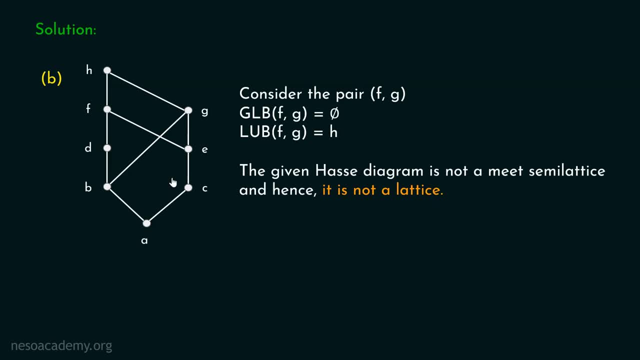 Okay, So this hash diagram is not a lattice. There is no doubt about this. Now let's consider this particular figure. Consider the pair F- G. Again, we will consider these two elements, F and G. Greatest lower bound of F- G is B. 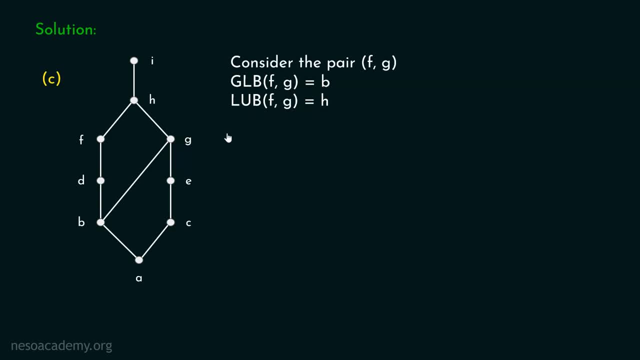 And least upper bound of F? G is H. You can see that the greatest lower bound, the point where they meet at first, is B And the least upper bound of F? G is H. Right, Consider the pair D and E. 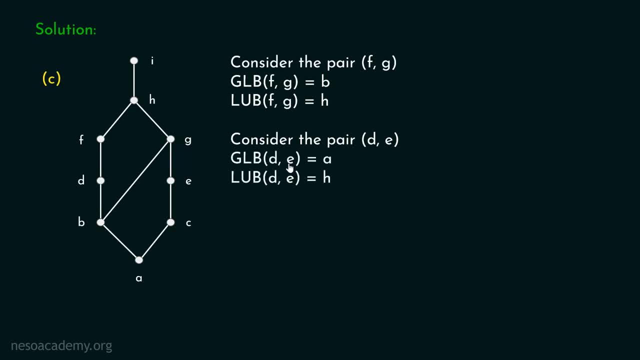 Consider these two elements, D and E. Greatest lower bound of D E is A And least upper bound of D E is H. Right, You can see that the greatest lower bound of D E is A And least upper bound of D E is H. 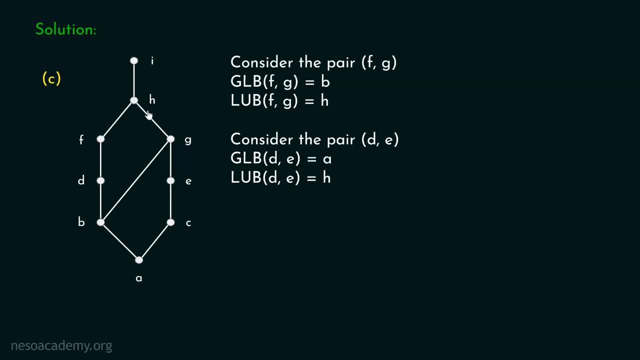 And least upper bound of D E is H. Right, And then you can also consider these two elements And you can clearly see that the greatest lower bound of B C is A And least upper bound of B C is G. 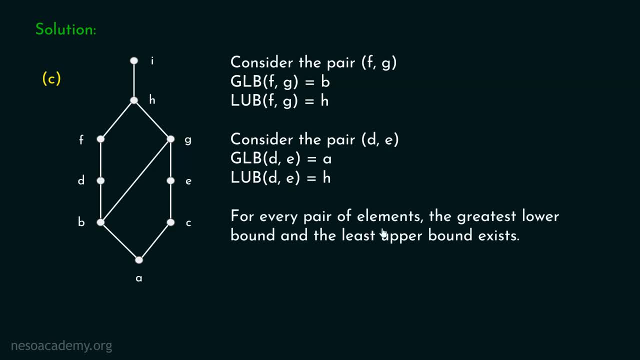 Right. It is clear from this fact that for every pair of elements, the greatest lower bound and the least upper bound exist Again. this is true. Therefore, the given hash diagram is a lattice. Right Now let's consider example three. 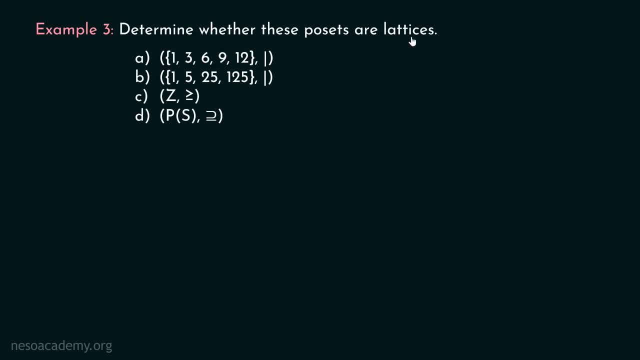 Determine whether these posets are lattices or not. Now the posets are available in front of us. We have to determine whether these posets are lattices or not. Let's identify whether these posets are lattices or not. 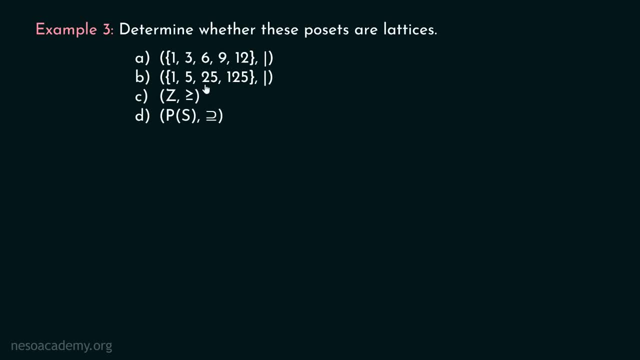 by first drawing the hash diagram for these posets, Because it is always easier to identify whether a given hash diagram is a lattice or not. So from these posets we will first draw the hash diagrams And then we will identify whether these posets are lattices or not. 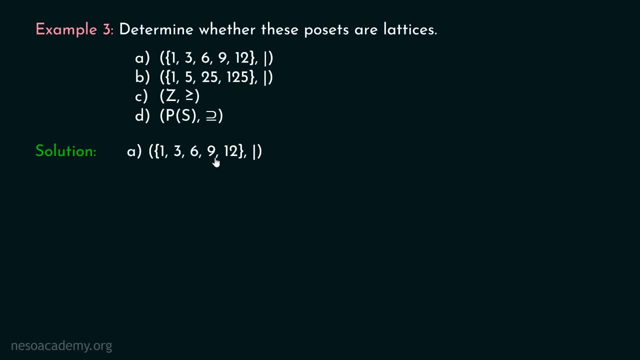 First, we will consider this particular poset, which consists of this set and this relation divides. Right Now let's draw the hash diagram for this poset. This is how the hash diagram for this poset looks like. Right, You can see that one has been placed at the bottom. 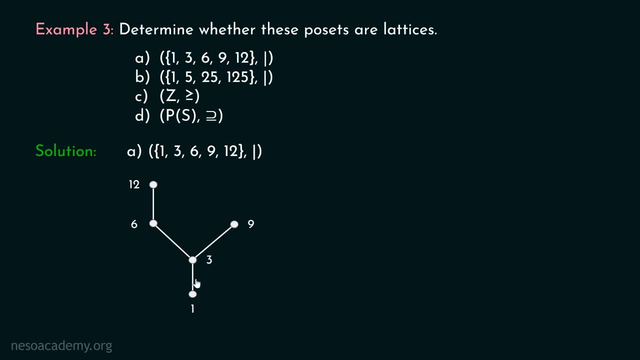 because one divides every other element. Then we have three, because one divides three, Then three divides six. So there is an edge between three and six, And three also divides nine. Therefore there is an edge between three and nine. 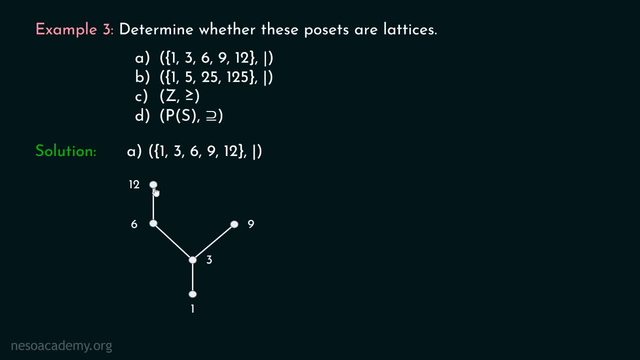 And you can see that six divides twelve. Therefore, there is an edge between six and twelve. Nine does not divide twelve. Therefore, there is no edge between nine and twelve, Right? So this is our hash diagram. Now let's identify whether this is a lattice or not. 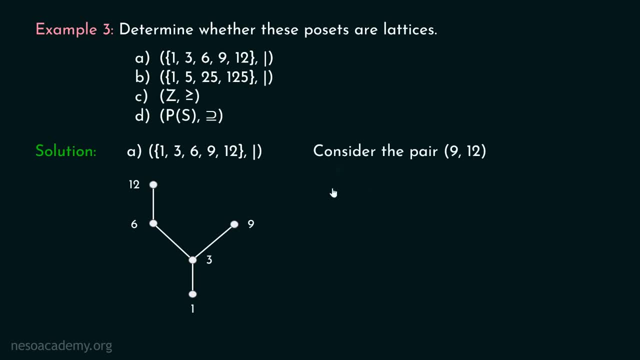 Consider the pair. Let's consider these two elements. You can see that the greatest lower bound of is three, Nine comma twelve. We have to consider these two elements. The greatest lower bound is three And least upper bound does not exist. There is nothing above nine and twelve. 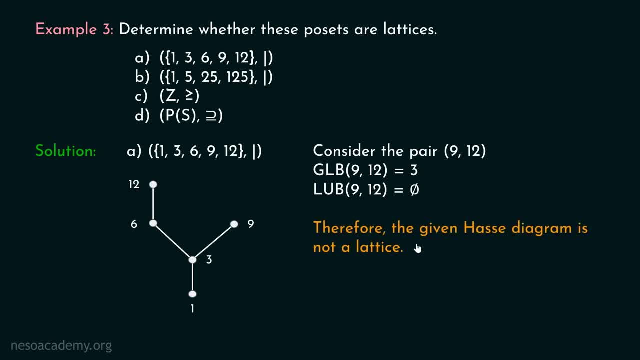 They do not meet at any point. Therefore, it is clear that the given hash diagram is not a lattice. There is no doubt about this. Let's consider this particular poset, And it is quite straightforward to draw the hash diagram for this poset. 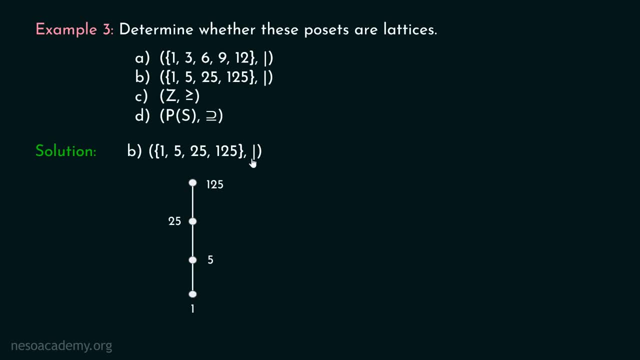 This is how it looks like. Obviously, one has been placed at the bottom. Again, we have a divides relation. Right. One divides five, Five divides twenty-five, And twenty-five divides one twenty-five. This is a total order, Isn't that so? 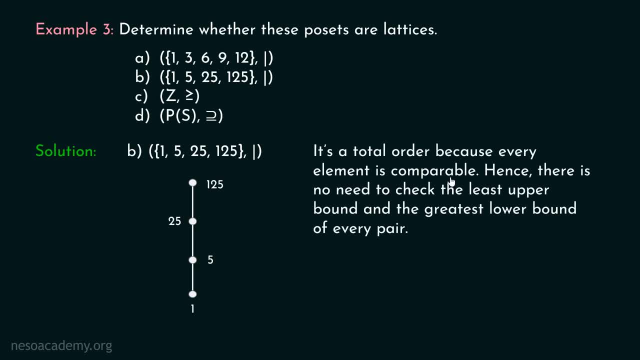 Here you can see it is a total order because every element is comparable. Hence there is no need to check the least upper bound and greatest lower bound of every pair. There is no need to check Because this is a total order. Every element is comparable. 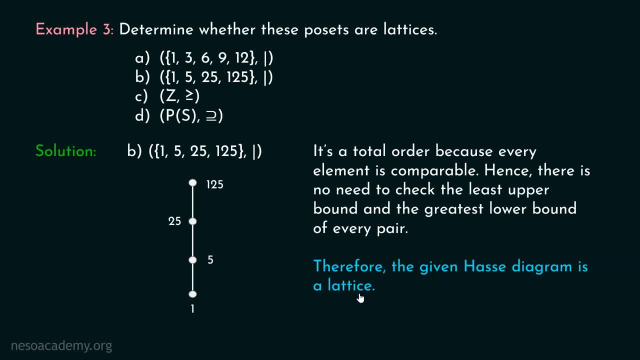 Hence we can say the given hash diagram is a lattice. There is no doubt about this. Every element is comparable. There is no incomparable element in this hash diagram. Therefore, the given hash diagram is a lattice. Let's consider this poset. 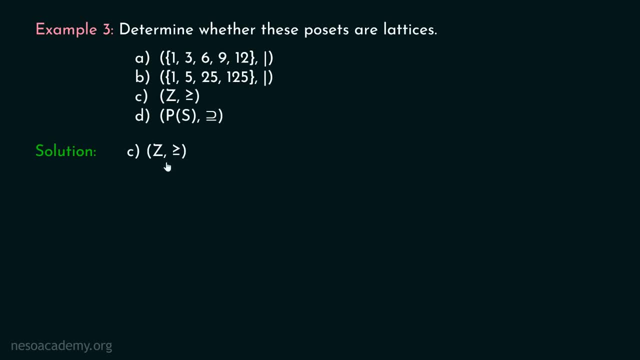 Z comma. greater than or equal to Z means set of integers, And we have greater than or equal to relation. Again, we got a total order, But this time we have an infinite lattice Right. It is a total order. Therefore, the given hash diagram is a lattice. 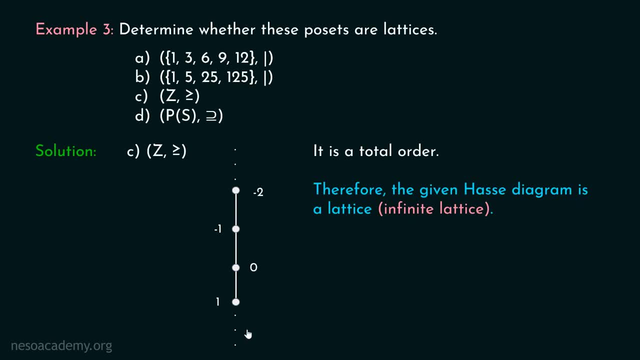 But this is an infinite lattice, A special type of lattice. You can clearly see we are talking about set of integers And we have a greater than or equal to symbol over here. Zero is greater than minus one. Minus one is greater than minus two. 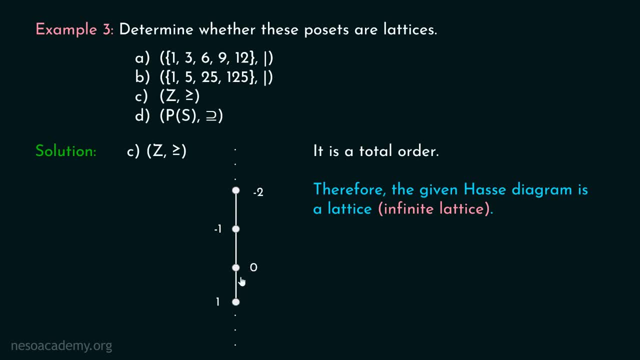 And so on. Similarly, here we have: one is greater than zero, Two is greater than zero, And we have more elements over here. It is clear that the given hash diagram is a lattice, Because it is a total order. Every element is comparable. 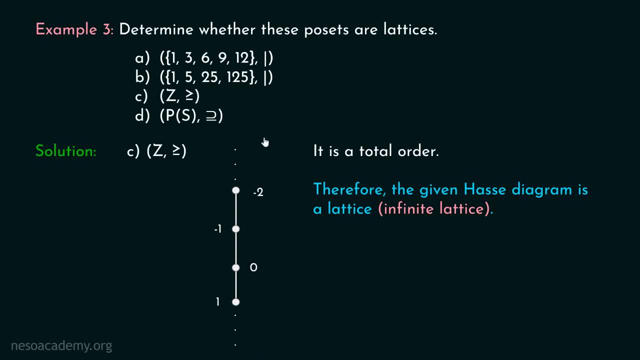 But this is a special type of lattice called infinite lattice. Fine, Let's consider this particular poset. Here we are talking about power set of some set S. Okay, Some set S is nothing but some set Okay, And we have this superset symbol. 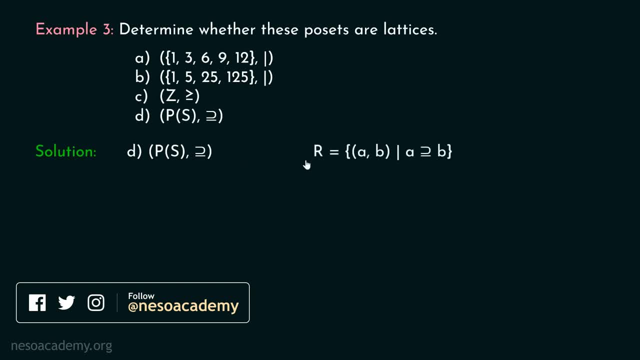 Okay, Instead of having a subset symbol, we have a superset symbol. Let's say: according to this, poset R is nothing but set of all ordered pairs, such that A is a superset of B, Right. Let's say: R is defined on power set of set S. 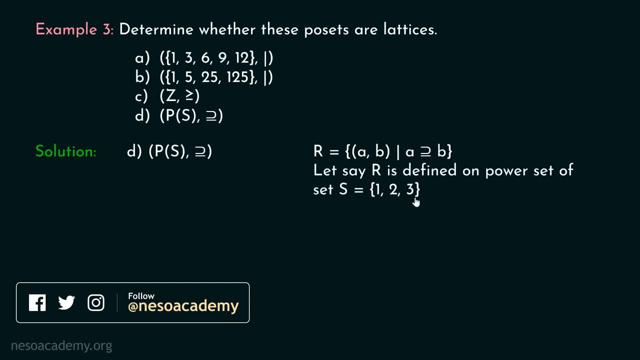 Which is nothing but one, two and three. Set S consists of these elements: one, two and three. This is some example. Let's consider some set S Right. Obviously, the power set of this set is nothing but five set with these elements. 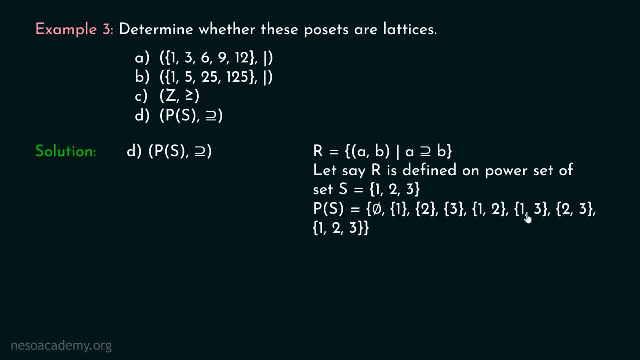 one, two and three. Then we have set with two elements, one comma two, one comma three, two comma three. And then we have a set with three elements: one, two and three. Right, This is power set of set S And obviously relation is defined. 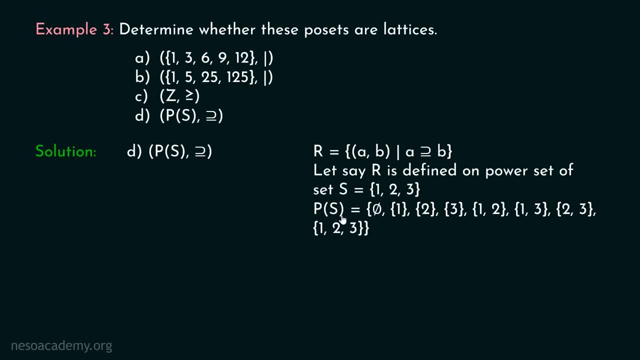 on power set of set S. Now, what is the bottom most element of the hash diagram? Obviously, this element would be the bottom most element of the hash diagram, Because here the symbol is superset symbol One, two and three. This particular set is: 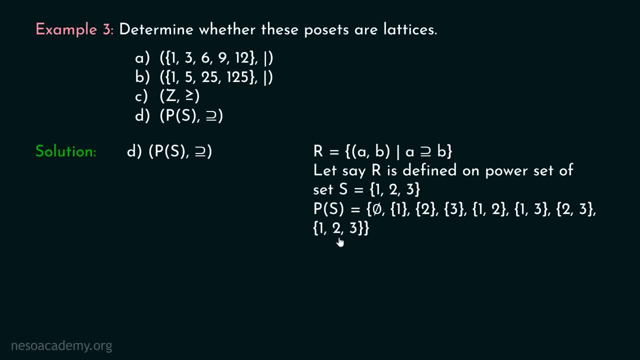 a superset of every other set. Therefore, we can place it at the bottom most place, Then after that we can place all these elements above this set. Right, You can see that one, two, three. this particular set is a superset of these three sets. 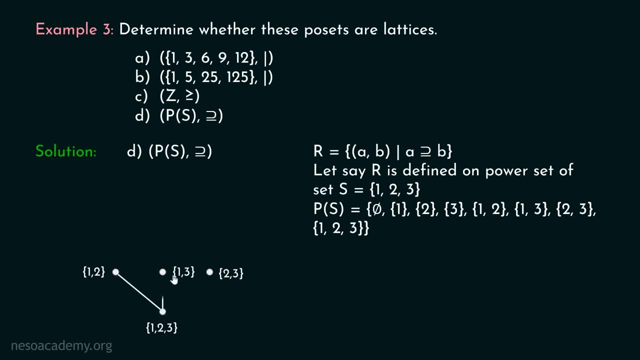 Therefore, we can draw an edge between this vertex and this vertex, this vertex and this vertex, and this vertex and this vertex. After this, we can place these three sets above these three sets Right, And we can draw an edge between this vertex and this vertex, this vertex and this vertex. 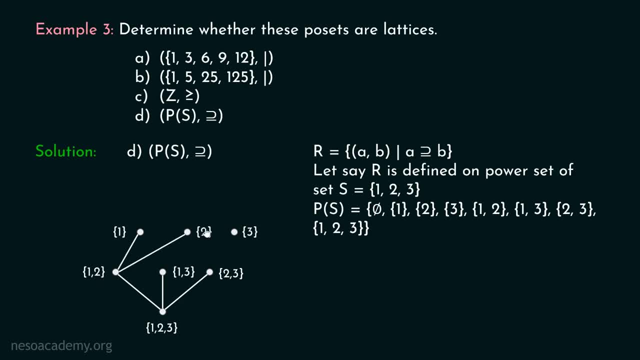